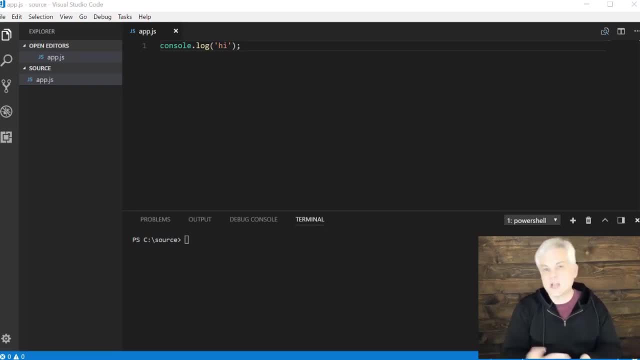 All right, And then we'll also then write JavaScript code that will execute in the context of a web browser, And we would expect for that code to be able to dynamically interact with elements- HTML elements- on a given web page. All right, But we might also use JavaScript to write video games in an environment like Unity, for example, and be able to author and control the various objects on screen and their animation and their interaction, and so on. 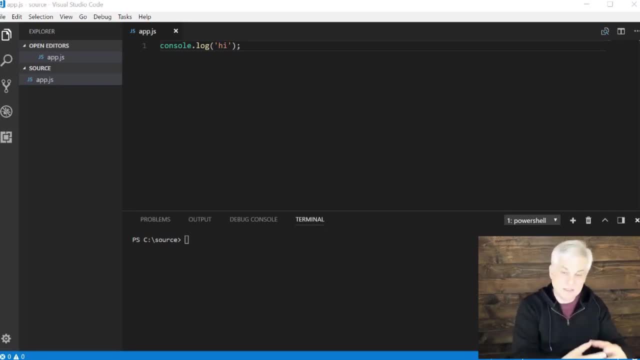 So what I'm trying to get at here is that there's a difference between the language itself and then the environment that it runs inside of, and we need to be aware of that, that those are two separate things, even though sometimes they feel like they're not. But we might also use JavaScript to write code for a web browser. So what I'm trying to get at here is that there's a difference between the language itself and then the environment that it runs inside of, and we need to be aware of that, that those are two separate things, even though sometimes they feel like they're not. 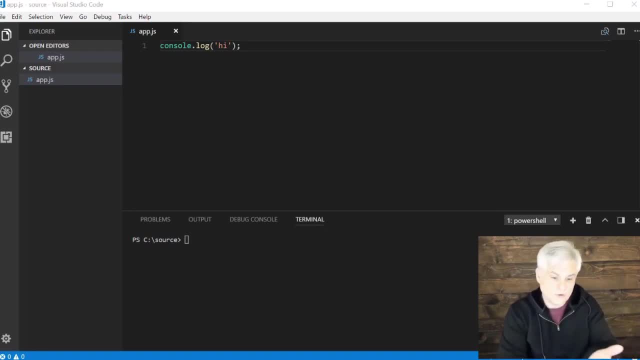 But we might also use JavaScript to write code for a web browser. But we might also use JavaScript to write code for a web browser. They feel like one thing, In this case console, for example. the consolelog function is provided to us by Node. 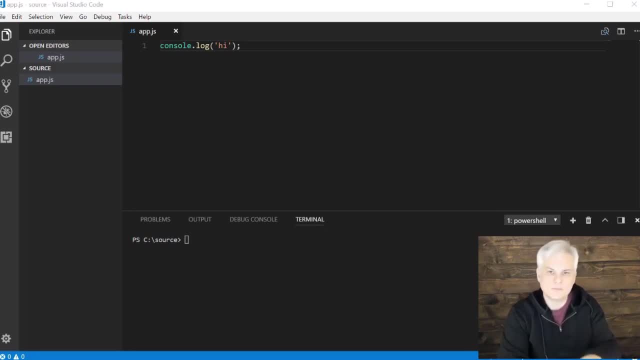 It allows us to tell Node that we want to print something to the command line, like we did just a moment ago. Now there's also a consolelog function in most web browsers and it allows us to print little debugging messages or console messages that can only be viewed inside of a web browser whenever we have a web browser. 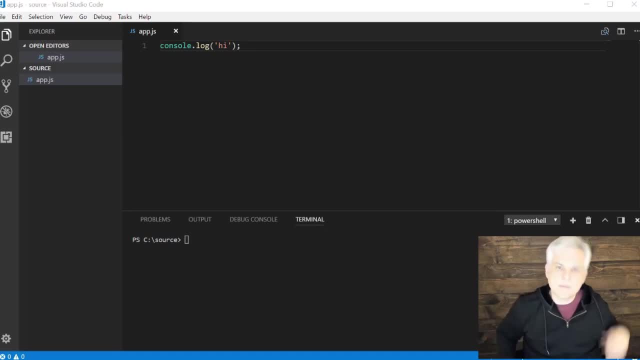 Whenever we have the developer tools open, and we'll see how to do that much later in this course, once we start building web pages and JavaScript that can interact with them. But at any rate, let's get back to the matter at hand here. 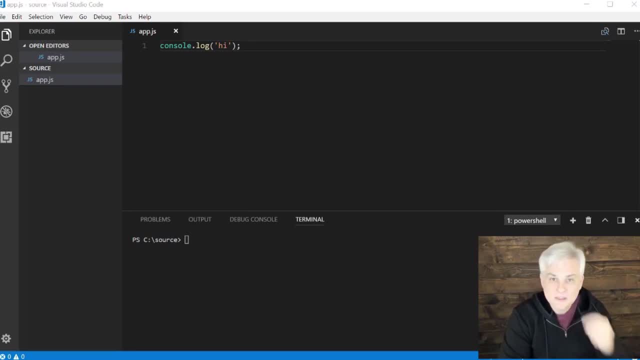 If I write my JavaScript incorrectly, then the runtime, whether it's Node or a web browser, won't be able to compile it and it'll give us an error. And so JavaScript is similar to English in so much that JavaScript has a syntax, and it has a proper syntax versus a syntax that's incorrect. 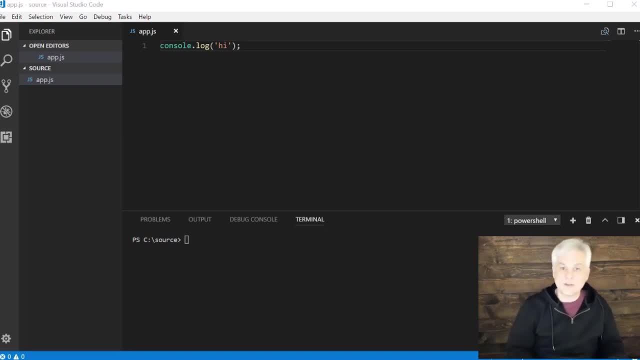 So if you've ever taken an English class, you'll know that there are parts of speech that you're supposed to use punctuation at the end of a sentence to indicate the end of a complete thought. There are nouns and verbs and adjectives and adverbs and propositions and all these sorts of things, right? 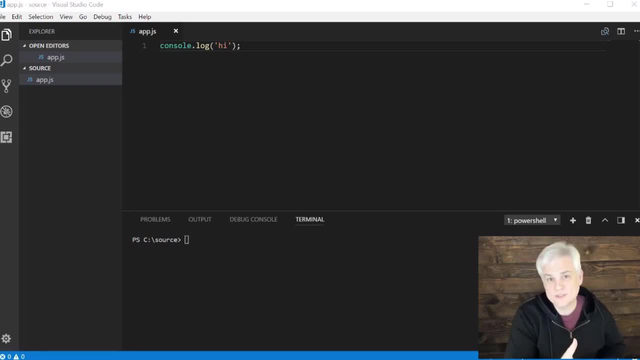 And so You know, in general terms, the same thing is true with JavaScript. There are parts of speech. We'll talk about those, And so you will be learning a new language, starting with your ABCs and with, I guess, vocabulary words, so to speak, and then to move on to authoring sentences that are complete thoughts and then stringing those sentences together into paragraphs in order to accomplish some higher-level task. 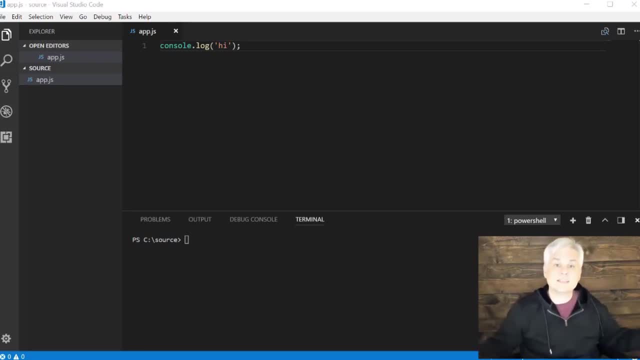 And even kind of arranging those paragraphs together All right. So hopefully that analogy will serve you well as we get started here. Our goal, as we get started, is to author JavaScript statements, And a statement is basically just one complete instruction. It's like a sentence in English. 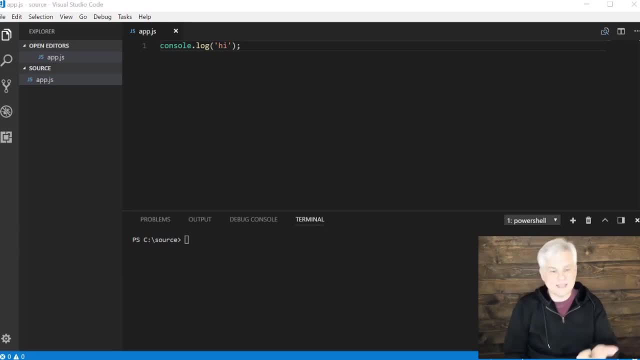 And each JavaScript file that we create, like this appjs, it'll contain one or more JavaScript statements that we'll execute in sequential order from time to time, top to bottom, at least usually, And I'll talk about the exception to that as we get further. 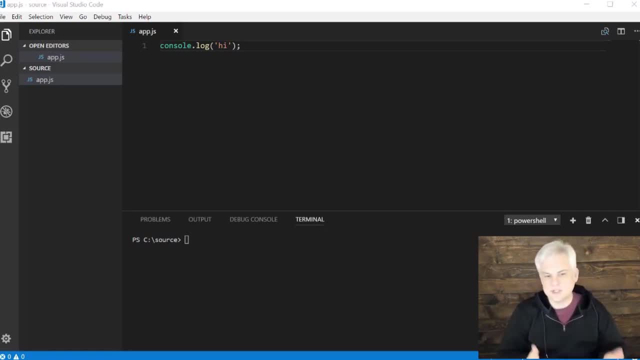 into this course. But there are some other similarities between JavaScript and English. For example, there's an end of line character. I was very, very specific about adding that semicolon at the end of our statement And that just is an indication to the compiler that this is a. 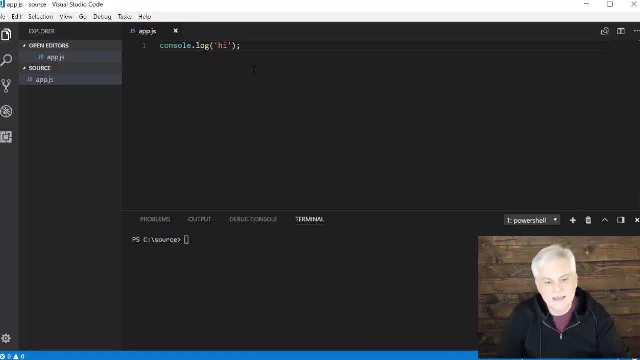 complete thought and it should be carried out as is All right. Now we also see that we have our statement all on one line of code And, generally speaking, as we're getting started, we're going to write our JavaScript statements one per line. Now we'll bend those rules as some 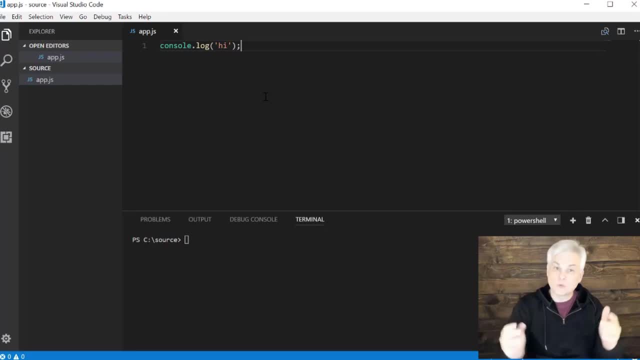 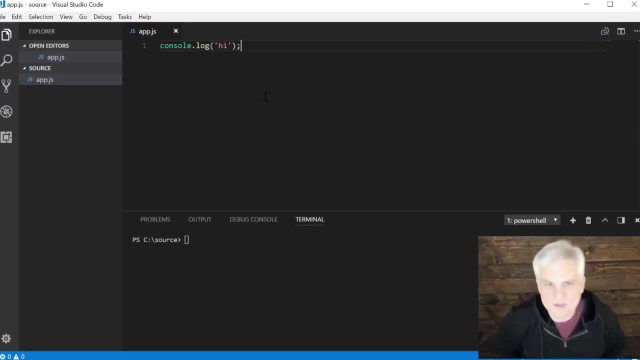 It can deal with a set of lines, But we're not going to write our single line for a given statement. But be that as it may, we're going to try to strive at the beginning to write one statement per line in our files, And a statement usually consists of one or more expressions. 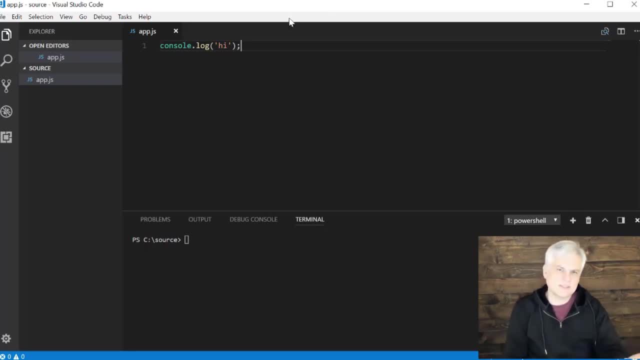 So we'll talk about expressions a little bit later. But this particular expression is essentially just executing a function that's built into Node. It's the log function. It belongs to an object called console. We'll talk about objects and functions a little bit later here. 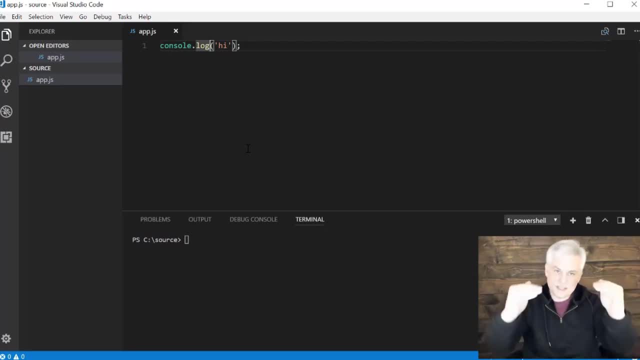 And we execute it by using operators, Those in this particular case, this is the function invocation operator or the method invocation operator. It's those open and closing parentheses, And we can even then pass in what are called arguments to those functions. So you can see. 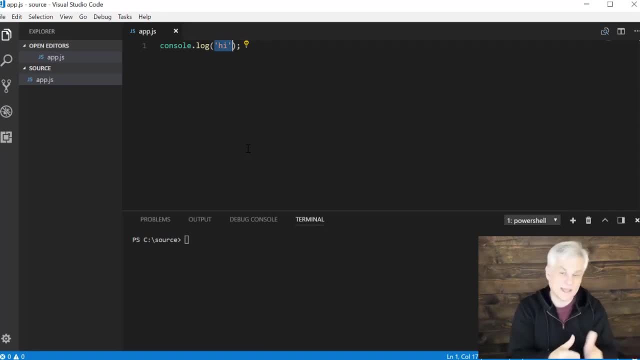 that each little piece of this has a name and it has a role to play in creating our functions, And we'll learn more about that as we move on here. One thing to note is that JavaScript is case sensitive, And this trips up a lot of people to begin with. That's why I was very specific to 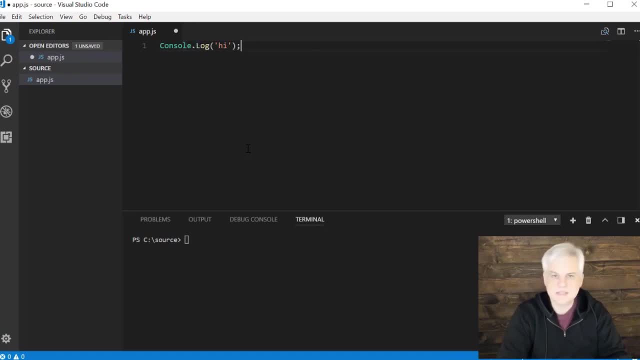 say: hey, don't accidentally or mindlessly use capital letters. Make sure everything is lower case. Let's see what happens if I were to save this work that I did here with the capital C in console and the capital L in log. Let's go node space app and hit enter And we get a reference. 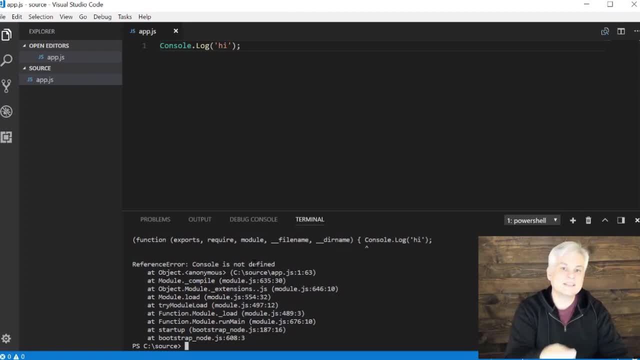 error: Console is not defined. It's not defined inside of node. Console doesn't exist with a capital C inside of node. It exists with a lower case C inside of node. The same thing is true with the function name log. Let's go ahead and I'll just use the up arrow on my keyboard. That'll give me. 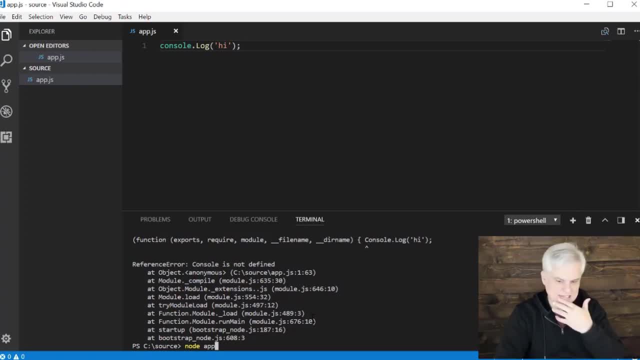 the last command that was used in the terminal. So again, node app, And I'm going to try to execute this little program again. And I get another error, This time console dot capital L log is not a function, That's true. It's because it's lower case L in log. 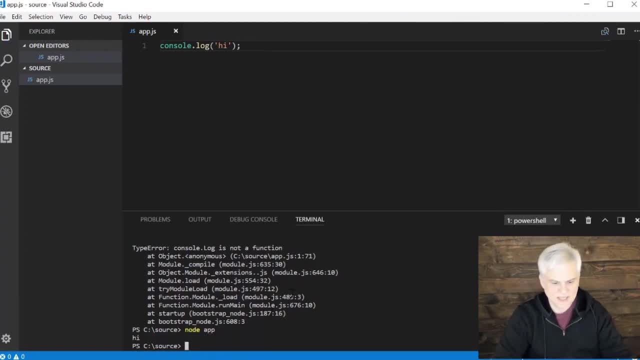 And I'll save that change And then we'll re-execute this And it will work. Now there are some things that, especially when your application is small, don't matter. So you might have accidentally left off that semicolon at the end and the application still runs. But that's a bad practice to 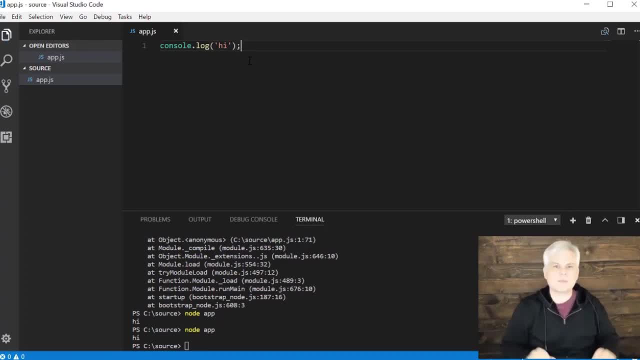 rely on that. You should always try to create properly formed sentences. Even though you could write an English sentence or a text message, you should always try to create properly formed sentences And you're relying on the person receiving that text message to understand what you're trying to. 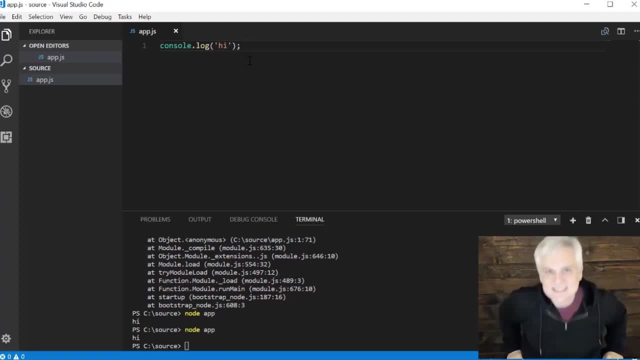 say. The computer doesn't work that way. It needs to know exactly what you're saying, And so you have to be precise. Precision is the key as a software developer. All right, So what I want to do here, as we kind of start wrapping things up for this first foray, I'm going to go ahead and 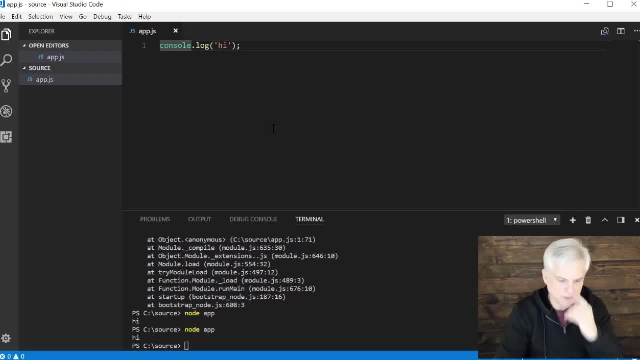 go into JavaScript. I'm going to comment out this line and add some new code below it and use that as kind of the next step beyond where we're at right now. So to tell the compiler to ignore a line of code, I'm going to add a code comment And here I use two forward slashes. I added also a space, but 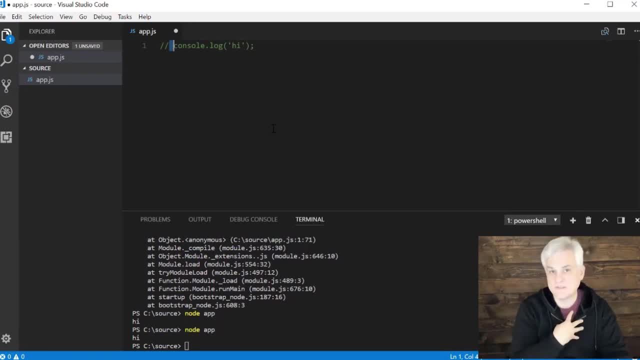 that was really just for readability's sake, so that myself, as a human, I can kind of make an easy distinction. because sometimes all these characters run together. I like adding a space between this. But these two characters say: forget everything on this line of code, Don't compile it, Don't try to use it. 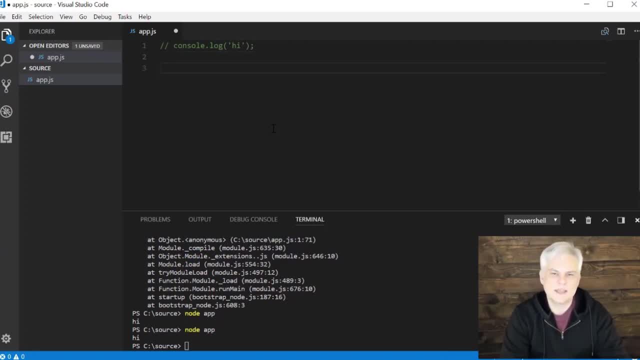 All right, And we'll see in a moment that there's another way to create code comments as well. But here let's create something a little bit more interesting. I'm going to say let x equal seven. I'm going to say let y equal. 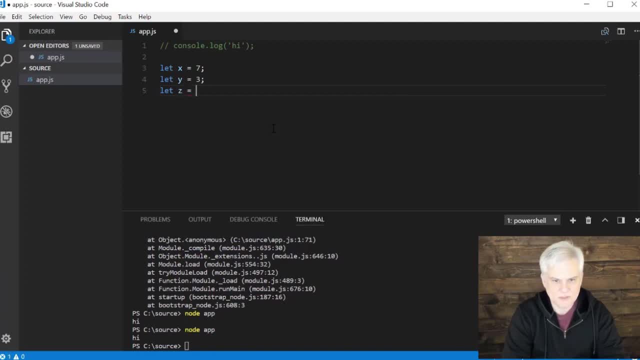 three. Let z equal x plus y, And then we'll do console dot log, And then I'm going to use the open and close parentheses, I'm going to use a single quote. I'm going to type in the word answer: colon space. 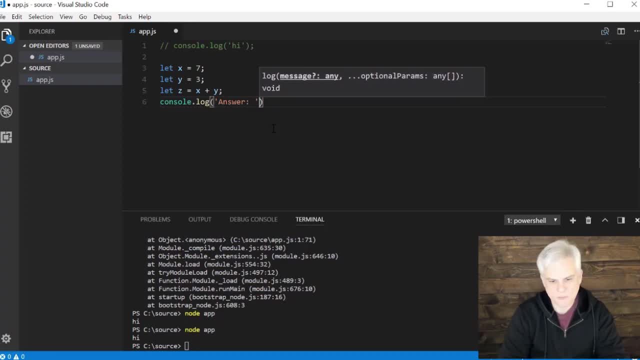 I'm going to go outside of that quote. So I'm going to go between the closing single quote and the closing parentheses And I'm going to make some space for myself in there. I'm going to use the plus key or the plus operator and the letter z. I'm going to go to the end of the line. I'm going to use the plus key. I'm going to use the. 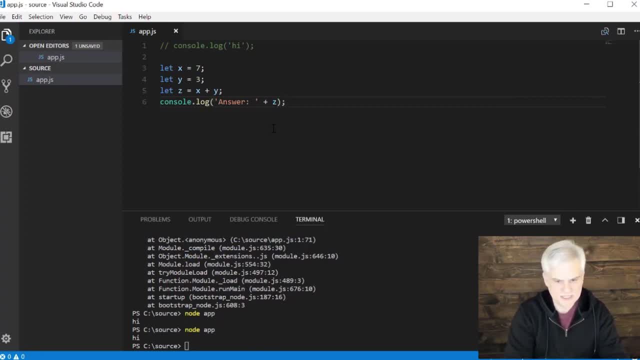 end of the line and use the end of line character, the semicolon. I'm going to save it all Now, before we actually execute this. what do you think this will do? What do you think will be printed to our console window? Do you have any? 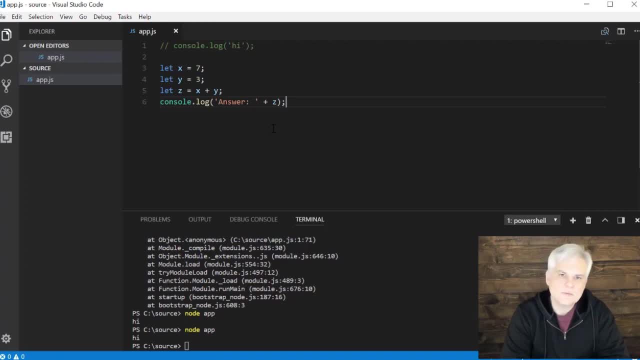 guesses. I'm betting that your background in math or algebra probably will lead you to the correct answer, And I think that your intuition in many cases is something that's important as you're learning JavaScript. It is human readable. It should be somewhat understandable. It might require a little extra explanation because there's some 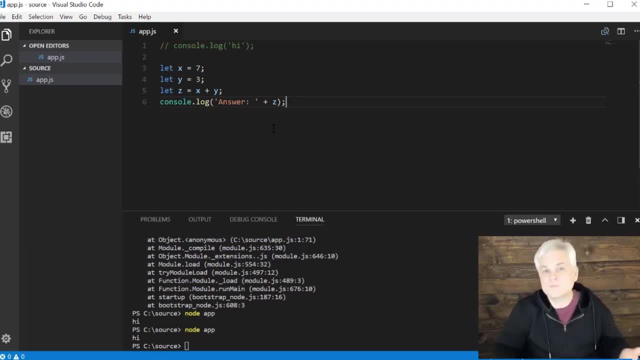 things that are not extremely obvious, But for the most part this shouldn't blow you away, And nothing we cover should ever blow you away. It just might require a little extra effort than you're normally used to putting into things, but by no means. 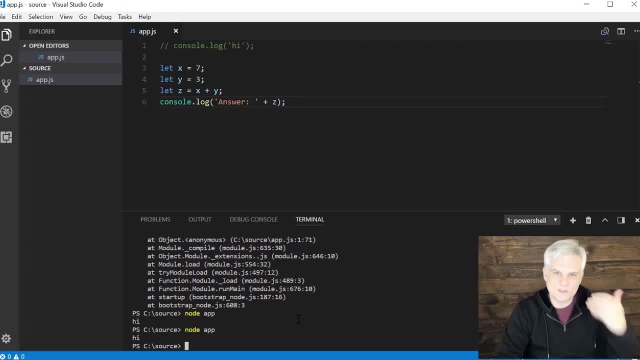 impossible, right? So just take some comfort that this is well-traveled ground and that, if I can understand it, I promise you can too. Let's run the application and see that we get started. Let's see if we get the correct result, which is answer, colon space and the number 10.. So how do we get that? Well, we have. 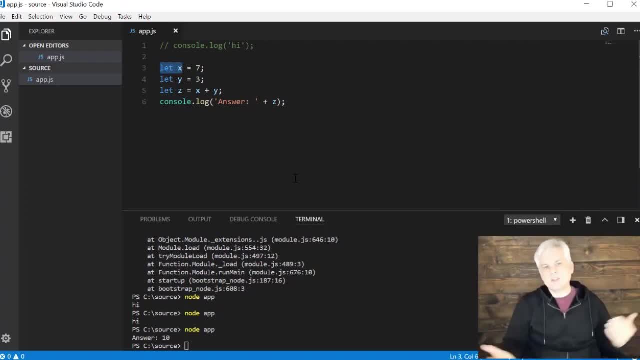 something here, let x. And even though, again, you're not a JavaScript developer or an advanced JavaScript developer just yet, I'm willing to bet that you understood that we were creating a variable, essentially a bucket, that could contain a value And 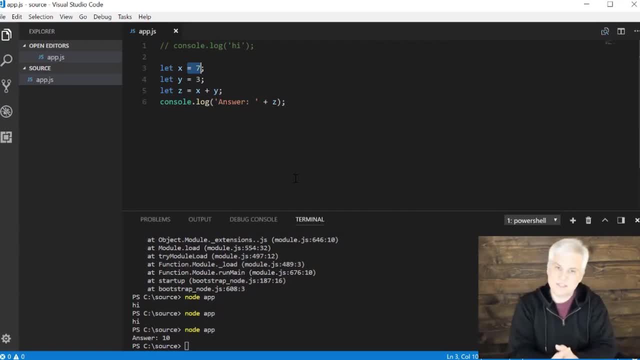 immediately, we set that variable equal to the value 7.. And then we did the same thing with the value of 3.. We put that into a different variable, a different bucket, called y, And then here we have an expression, an expression that will add two values together. What are the? 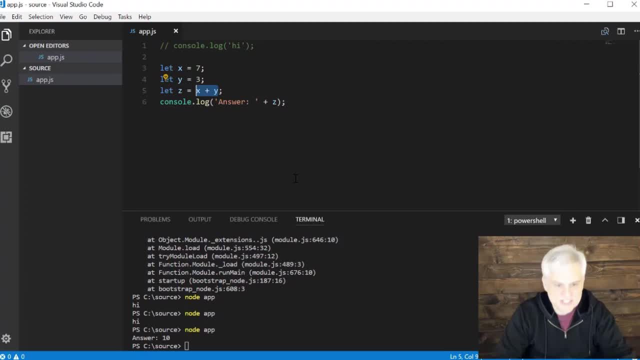 values inside of those variables x and y. Well, we just assign them in lines three and four, And we know that that probably means we're going to add those together to get the result of 10. And we assign that into a new bucket, a new variable. 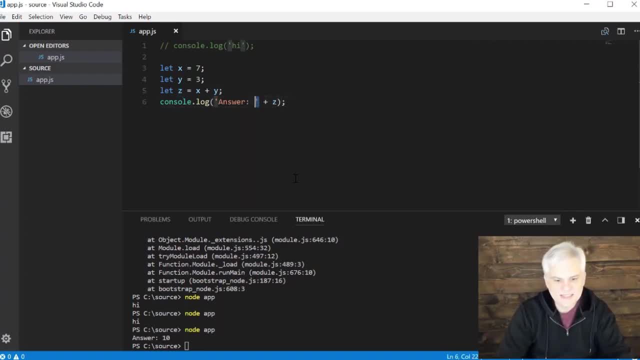 named z And then we merely print out that literal string, But then we also say: also append the letter or the value that's in z. Now, hopefully that made sense to you even before we ran the application. But you can see here that, for example, the plus symbol has has double duty.